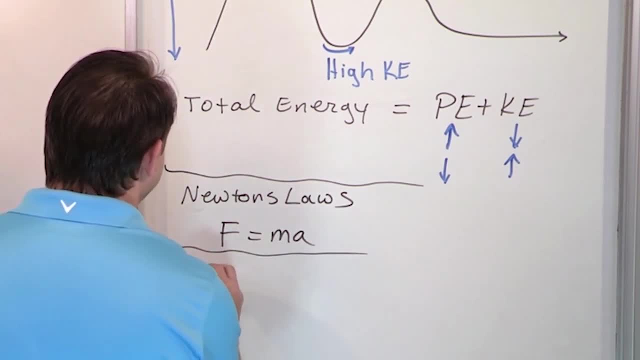 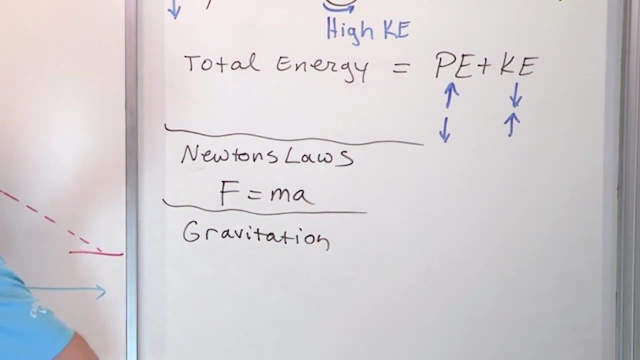 while and solve tons of different types of problems. we're going to talk about Newton's law of gravitation, which is a really big deal, obviously, because we live on Earth and there's gravity here. What does this mean, though? If we have a planet, we're going to call it Earth. 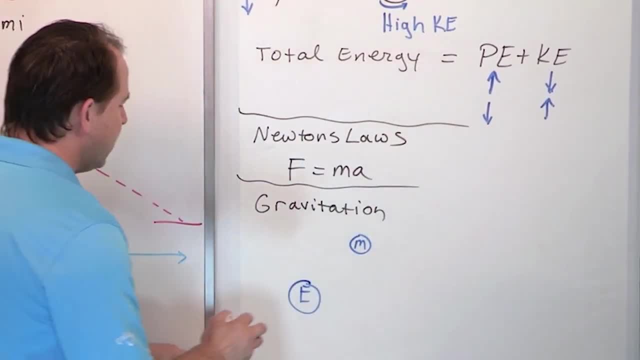 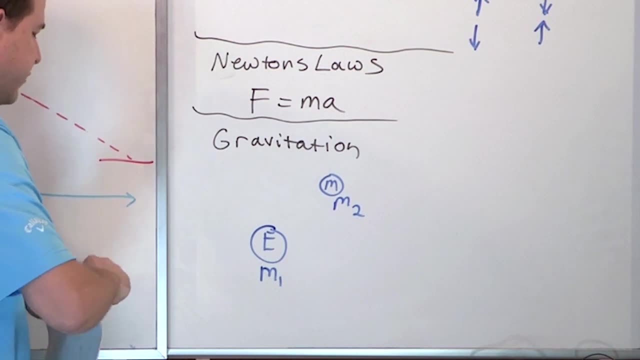 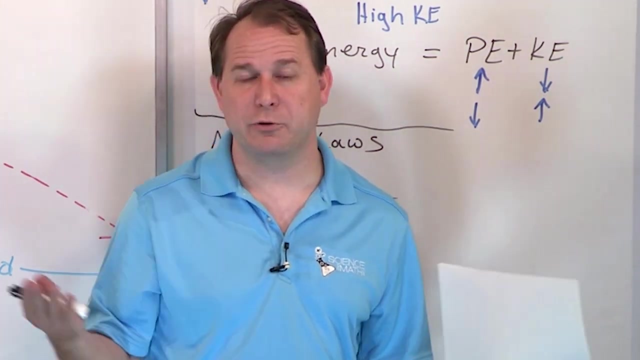 and we have a moon here, we call M. So the Earth has some mass, We call it M1.. And the moon has some mass, and we call it M2.. What Newton figured out is there's a force that exists between any two pieces of matter. It exists between you and your pencil. It exists between a lamp and. 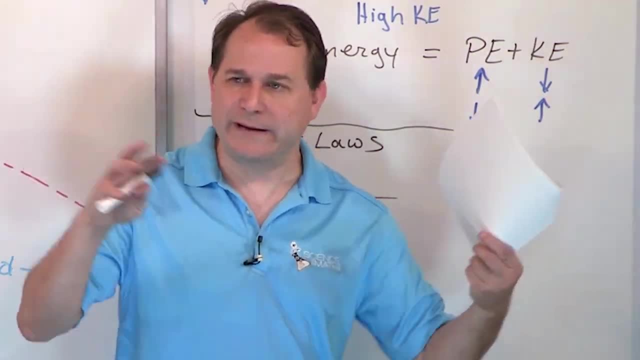 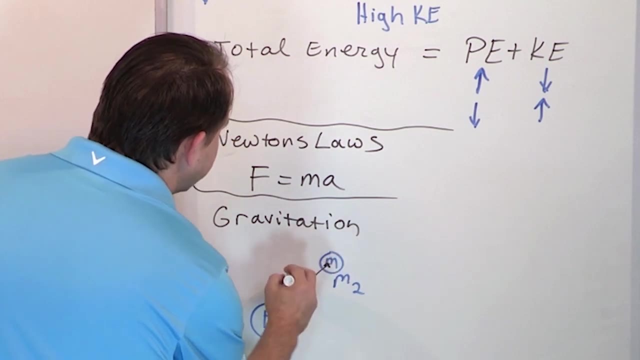 television. It exists between the Earth and the moon. Any two pieces of matter pull on each other with some force of gravity, And that force, if the distance between these two things we call R, that force of gravity- is equal to some number- G, which we'll talk about- It's called the. 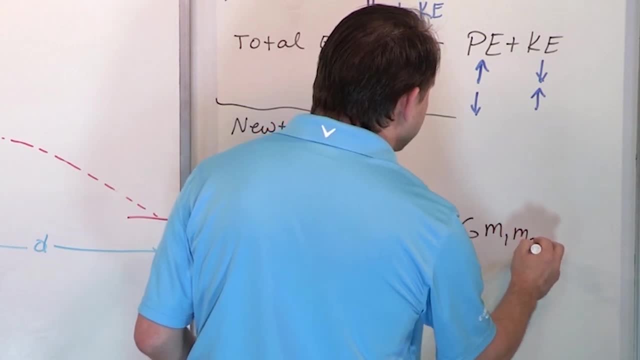 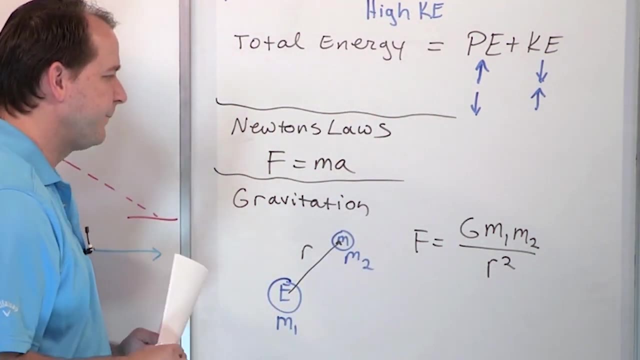 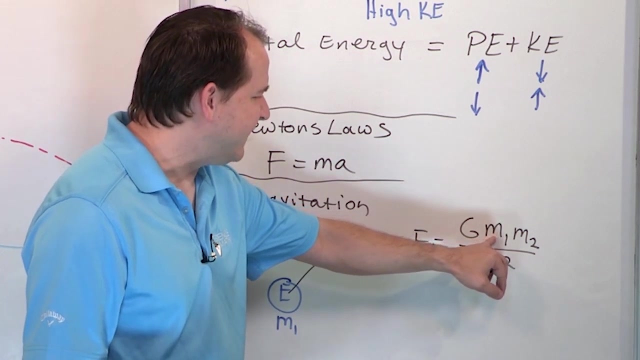 gravitational constant Time. mass 1 times mass 2.. So we're multiplying all the masses together, times G this number, And on the bottom it's the distance between them, but squared, So you might hear this called the inverse square law or something like this. So if the Earth's mass gets 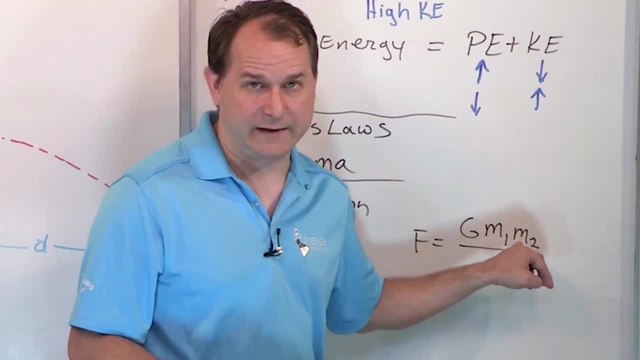 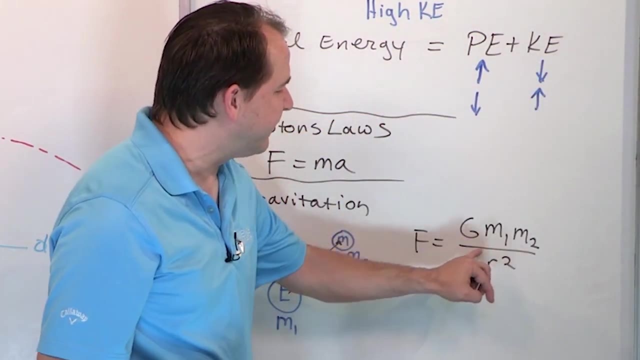 bigger M1, then the force is bigger. If the moon's mass gets bigger, the force is bigger. But if we increase the distance between them, like if we stretch out the Earth and moon even bigger, then, since it's in the bottom, we're dividing by M2.. And if we increase the distance between them, 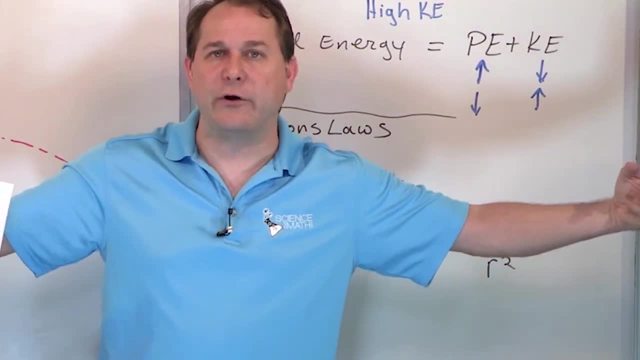 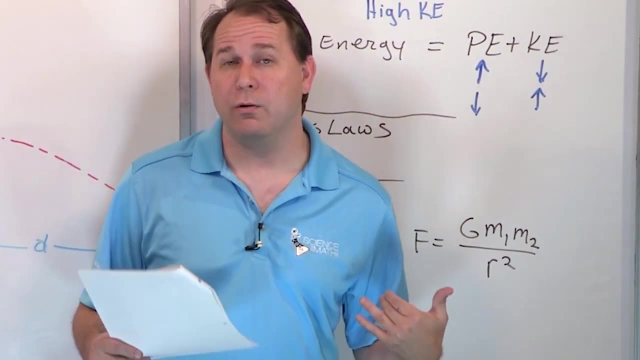 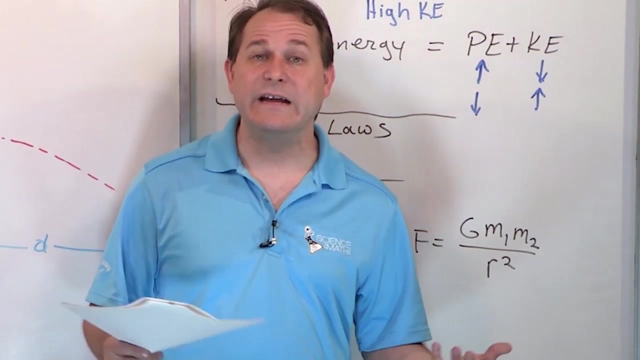 we're dividing by bigger numbers, So the force actually goes down as we make things get farther and farther apart. So this is called the universal law of gravitation. Now we actually know, now that Einstein, a couple hundred years later, released and invented his theory of gravitation And his 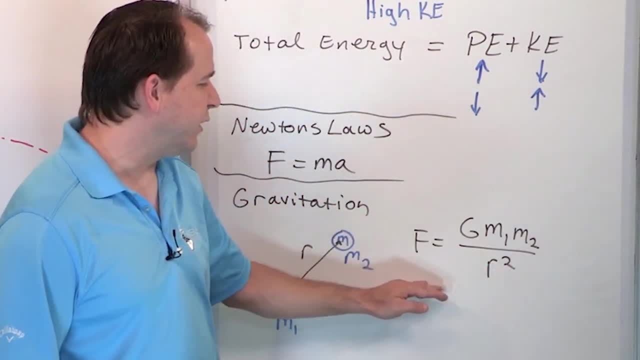 theory of gravitation is actually more correct than this one, But still this is a really good starting point to understand gravity, And we're going to solve lots of problems using Newton's form of gravity, because it's a whole lot simpler than Einstein's. 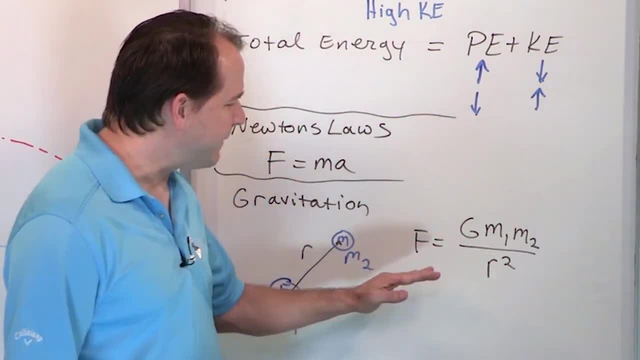 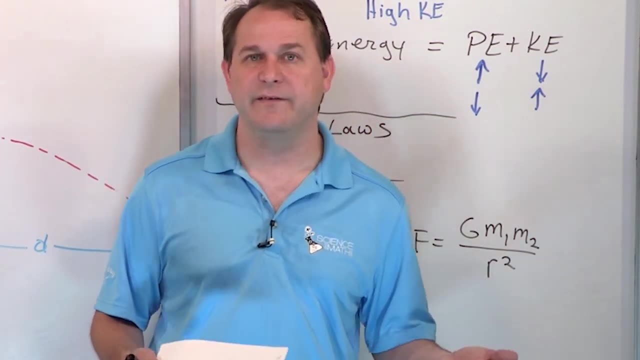 theory of gravity which is beyond the scope of this class. But just keep in mind that you know this was accepted fact for 250 years or so And now we know that it's not quite right in some instances. And in the early 1900s Einstein published a theory which totally reinvented. 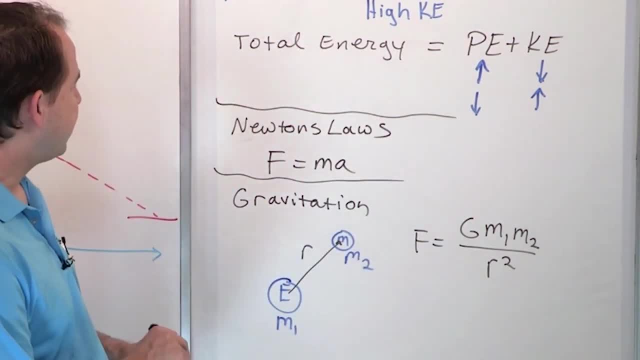 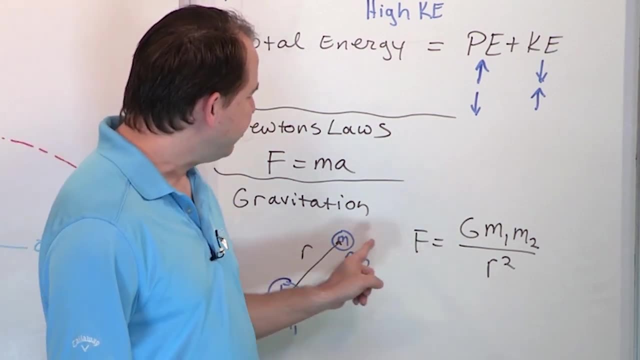 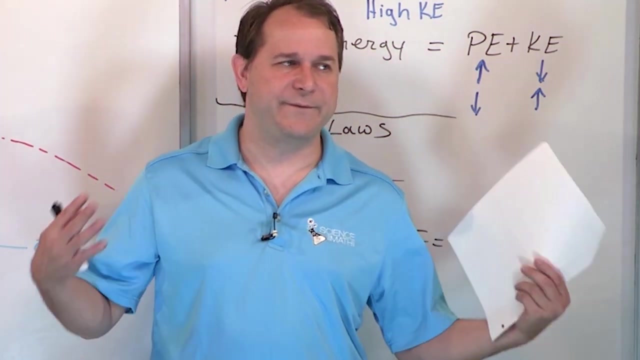 how we look at gravity completely. But you might ask yourself: if I push on something, it's going to accelerate. Then, if there's a force between the Earth and the moon here, shouldn't the moon come crashing in to the Earth? Shouldn't it come crashing into the Earth? Well, of course it should, Absolutely, And that's the 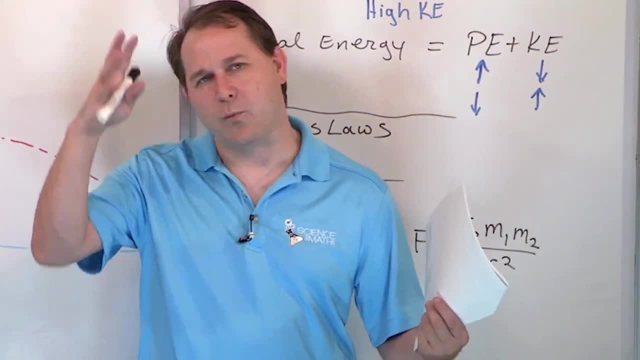 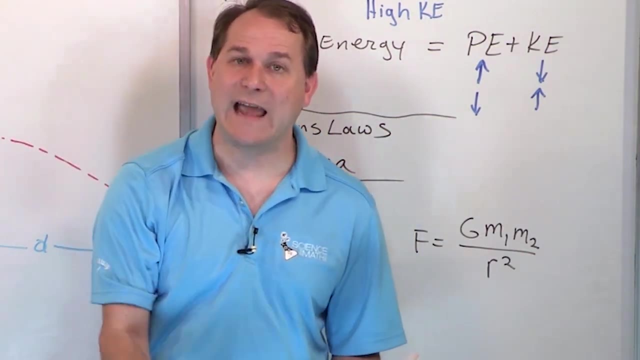 famous thing- you know, Einstein- I mean Newton- sitting under the tree and watching the apple fall and having who knows if it's true or not. That's the story. right. He realized that the Earth is pulling on the apple and the apple falls down. He realized maybe the Earth is pulling on. 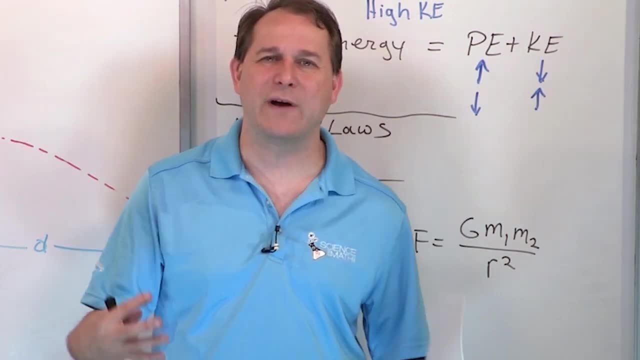 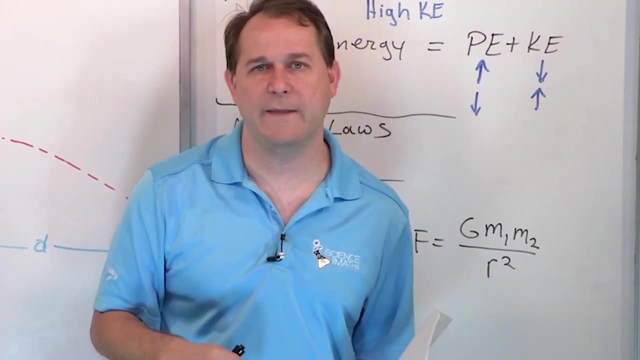 the moon with the same force. Well then, why is the moon not crashing down like the apple? That's the real question. But he thought, well, maybe it's possible that gravity is extending all the way to the moon and pulling on the moon. And he thought, well, maybe it's possible that gravity 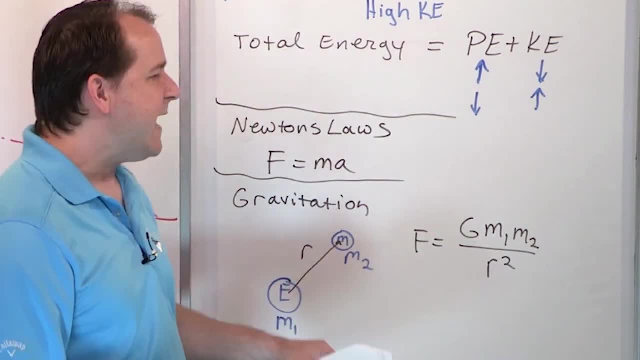 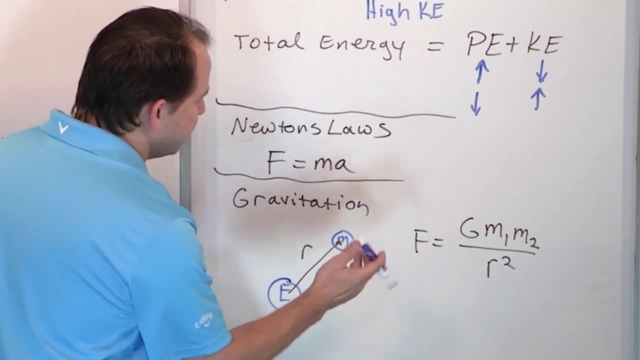 is pulling on the moon, And the answer to the question is it is pulling on the moon And if the moon were not moving, it would crash into the Earth. However, the moon is actually moving. It's moving sideways with some very high velocity V, So it's going around and around and around It. 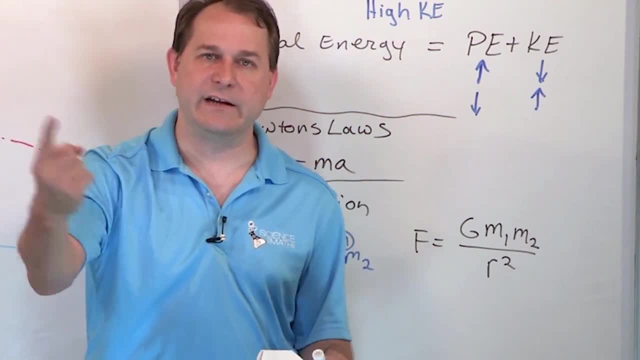 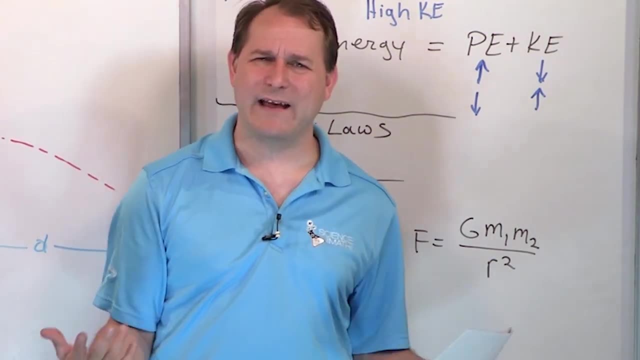 is being pulled in, but it's going so fast in the horizontal direction- for lack of a better word, that's called the tangential direction- that it never really hits the ground. And you say: how is that possible? Well, I have a little prop here. It's not a great. 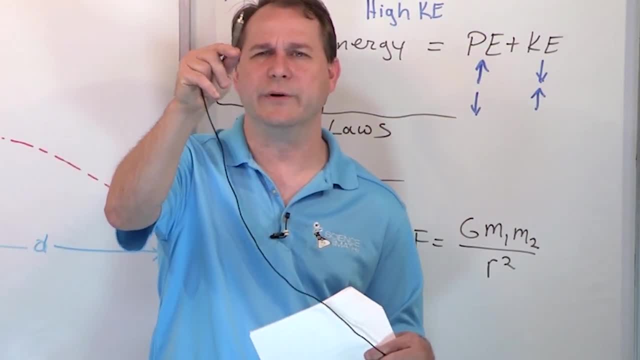 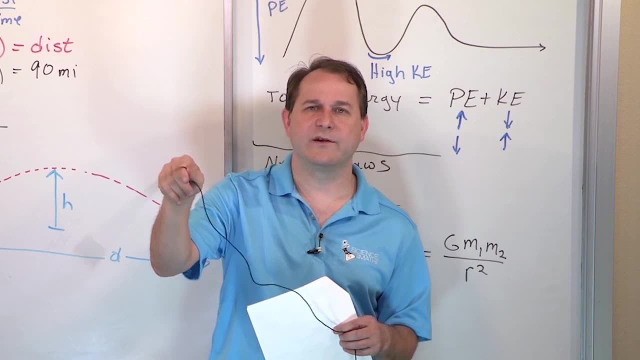 great prop, but it's a little prop. So this is like, this is like the moon here on the end of my little wire. Well, if I take this guy and start spinning it around, what happens here? Well, you see, it's going round and round and round and round, just like the moon is. But what am I doing? 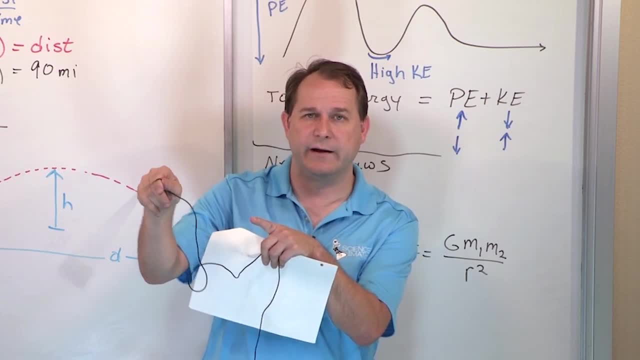 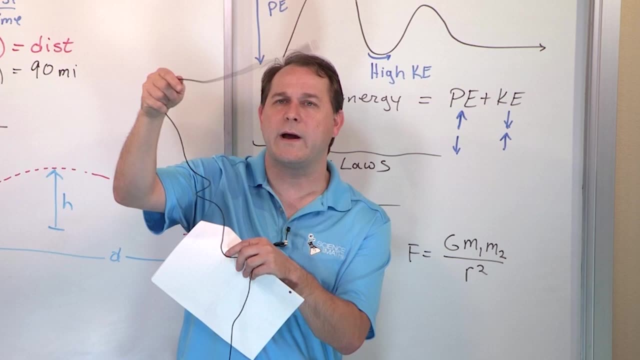 with my hand in the center. Look carefully, I'm actually pulling on this thing. So what I do is, when you start it off, you have to give, you have to start swinging it right, Like I'm swinging it, and then I get it to go around once And then I go. it gets to go twice And then I then once it's. 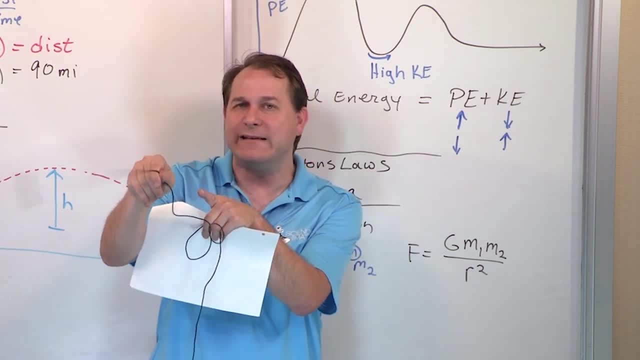 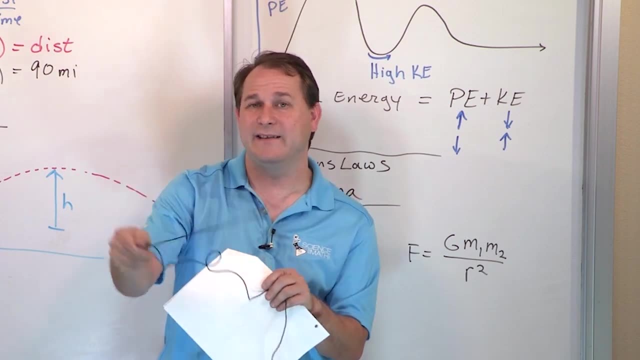 horizontal like this. I'm pulling on it, I'm pulling it straight into my hand, but it never hits my hand because I've given it a very fast speed horizontally like this, And that's basically the exact same thing happening with the moon. If the moon weren't moving at all, if it just stopped. 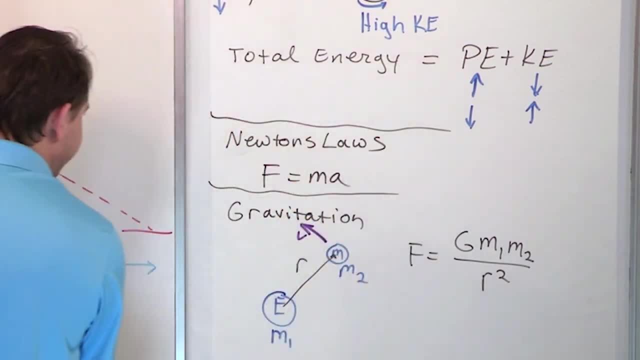 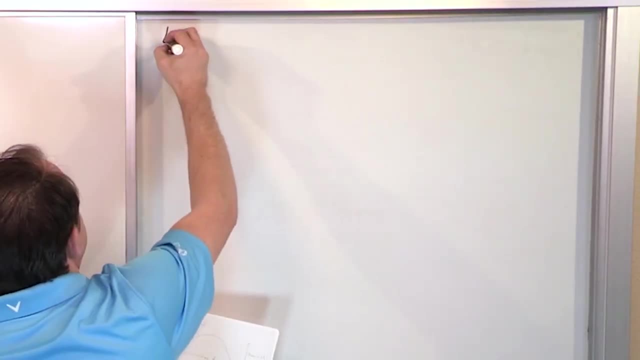 then it would accelerate straight down and hit the earth, But only because it's moving so fast horizontally can we escape that? Now? the next thing we learn in physics typically is the concept of energy, And I know that most everybody here has an idea. 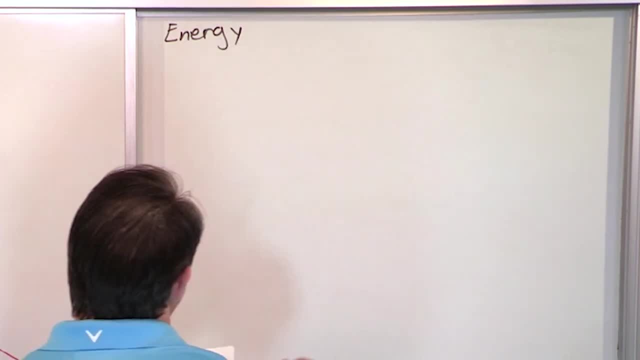 Of energy, But we're going to talk just to just a brief minute about energy. So the best way I can describe energy is- or at least one type of energy is- a roller coaster. So here's a roller coaster, very high hill and then comes down to the bottom and then a little bit like this, And then maybe 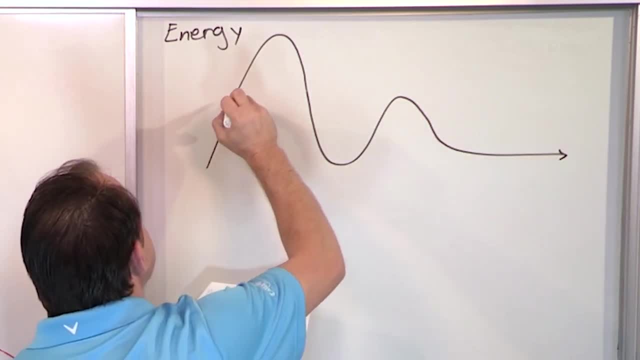 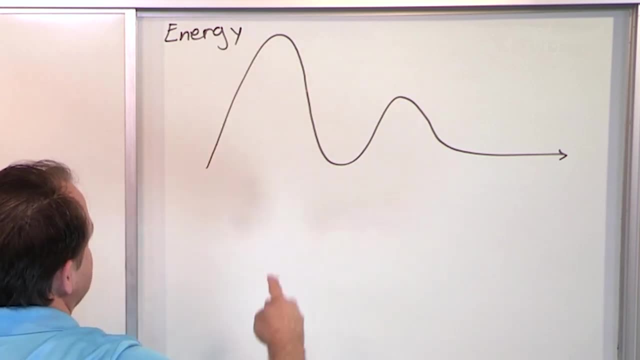 it just kind of does something like this: So there's a car, clink, clink, clink, clink, clink gets to the top, Very, very, very high right, At the very top of this very high mountain right. 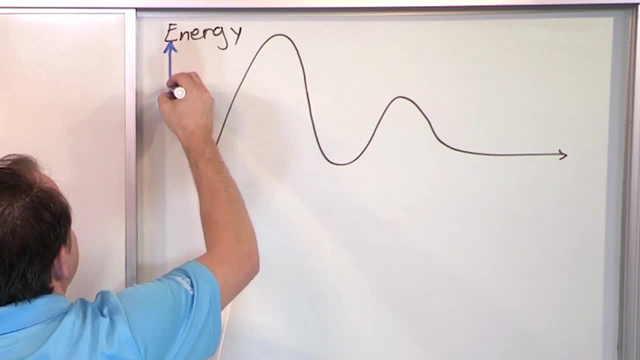 And then we say that it has a high potential energy. High potential energy. I don't have room to write out potential energy, But the reason it has potential energy at the top is because we're in a gravity field. So if you 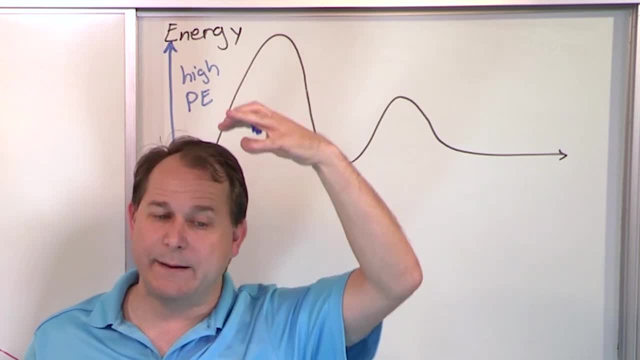 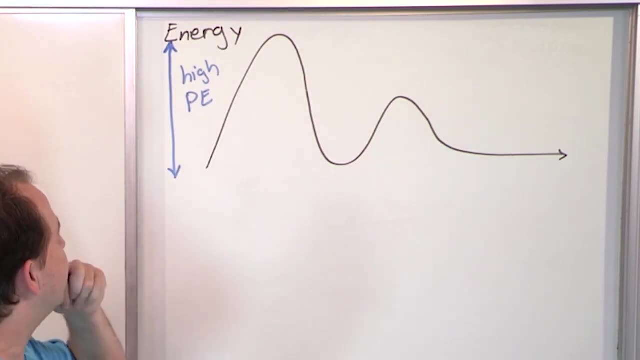 bake something very high off the ground if you were to drop it. it has a high potential to accelerate down to the ground and to hit the ground right. So to do something to hit the ground, to have to do some, impart some energy into the ground. So we say it has a high potential. 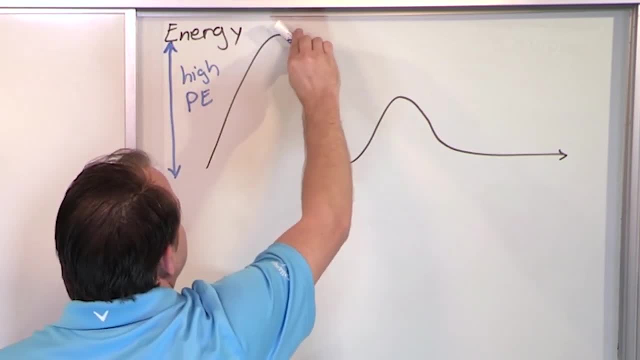 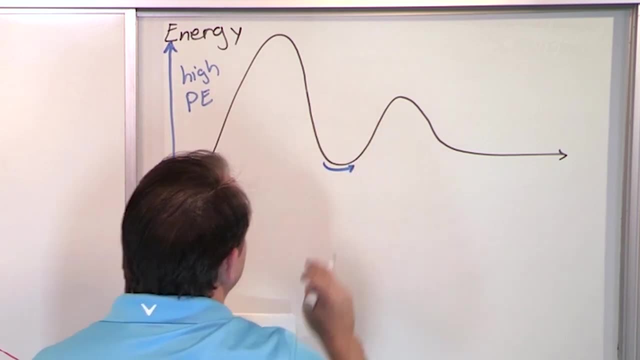 energy here. So what happens is the roller coaster goes to the very bottom and all of that potential energy you have because you're accelerating. when you get to the very bottom here, when the roller coaster starts to round the bottom down, there we say that we have a high kinetic energy. 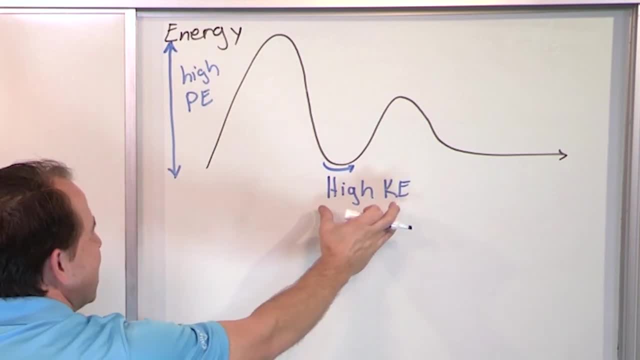 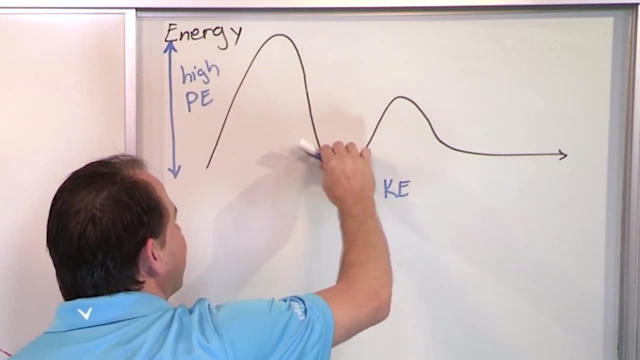 So we're going to learn a lot about potential energy and kinetic energy. Kinetic energy is how fast you're moving. It's the energy of motion. So you know, when you get to the bottom of the of the of the trough here in the roller coaster you're going fastest, Up, here you're going slow. 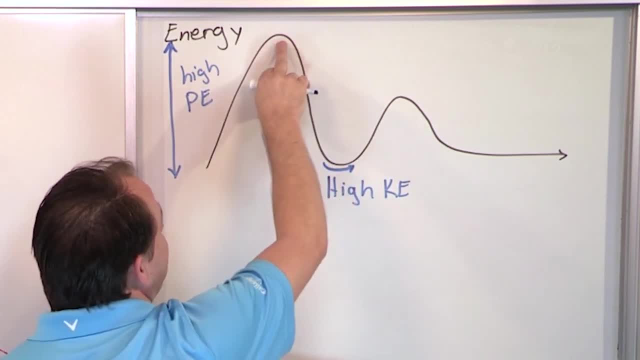 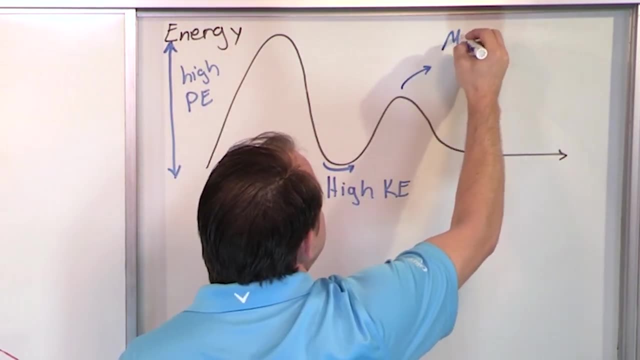 So you have very low potential energy here. I mean, sorry, high potential energy here, and it's all converted into kinetic energy. And then here over at this part, what do you have? Well, you have medium potential energy, because you are a little higher off the. 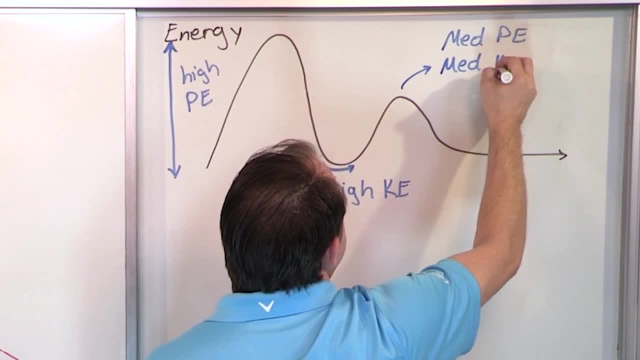 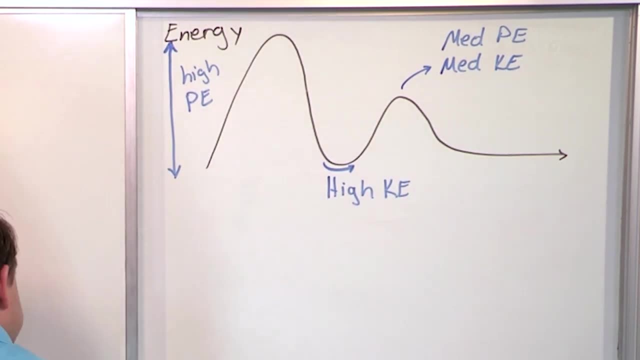 ground, but not as high as here, And you have medium kinetic energy. because you're not going quite as fast as you were down here, You bleed off some of the speed. So one of the big, big, big, big, big, big big things we're going to do in physics is we're going to talk about the total.